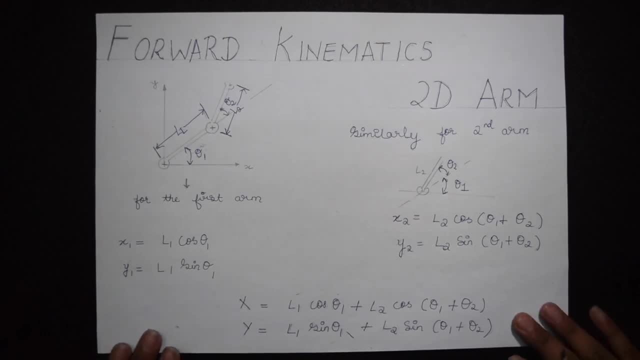 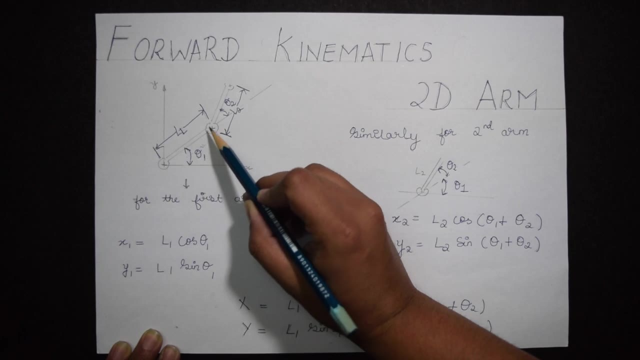 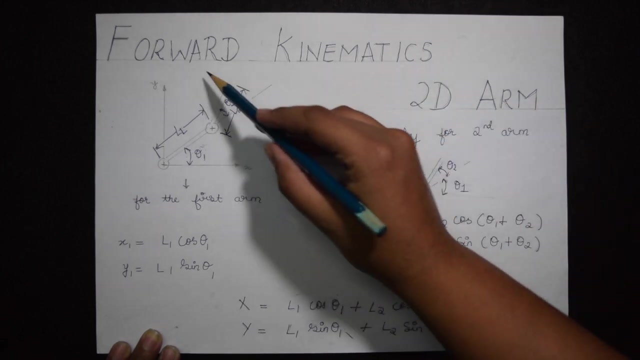 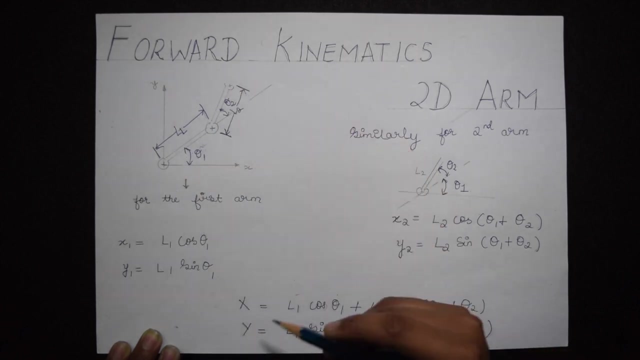 Forward kinematics refers to the use of kinematic equations of a robot to compute the position of the end effector from specified values for the joint parameter. So today we will be doing the forward kinematics of a 2D arm. Let's look at this arm. You can see that it has two arms: L1 and L2.. 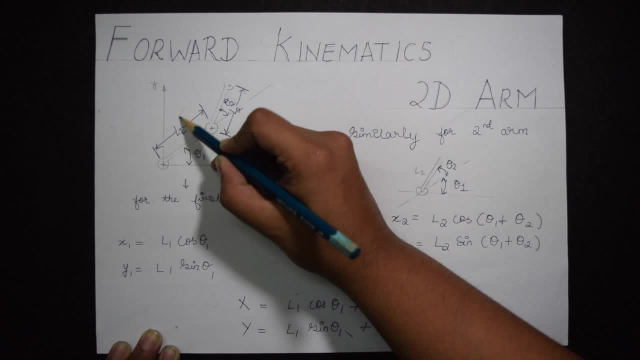 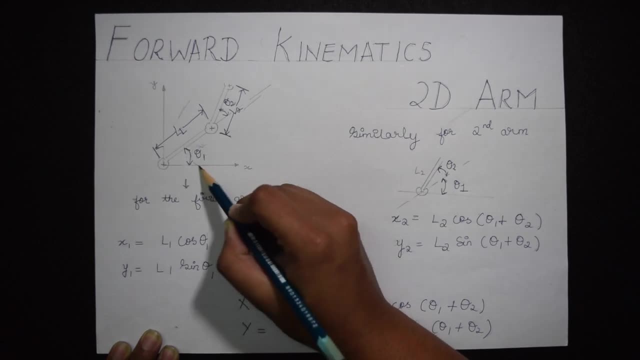 L1 is the length of the first one and L2 is the length of the second one. The first arm is at an angle of theta1 to the base and the second one is at an angle of theta2 from the first one. Now let's look at the first arm. 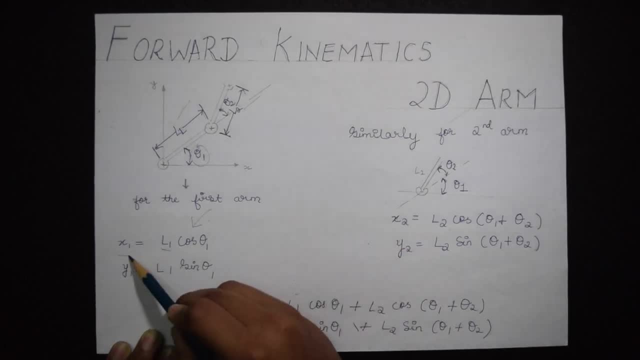 We see that we get the x1 component of the first arm as L1 cos theta. You know the maths right. So similarly for y1 and y2, we get the x1 component of the first arm as L1 cos theta. 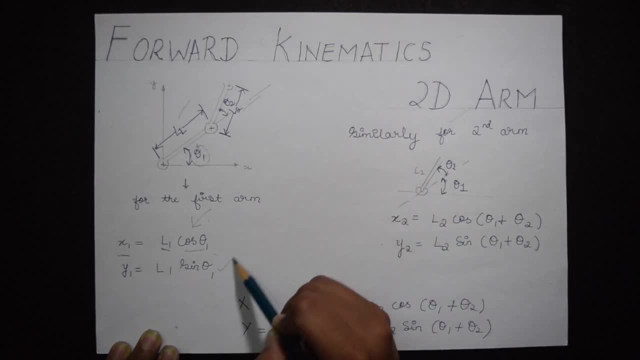 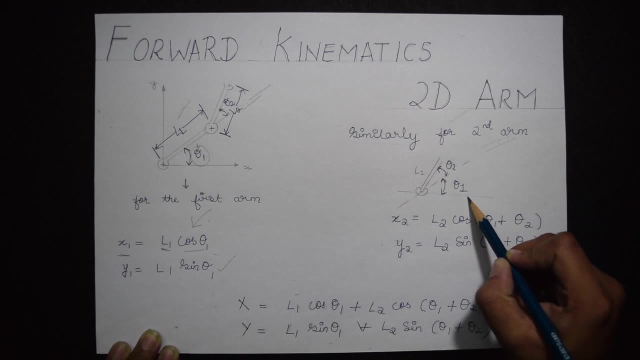 For y1, you will get L1 sin theta. The tricky part comes here. in the second arm We see that it is at an angle of theta2 from the first one. So if we look from the base it is at an angle of theta1 plus theta2.. 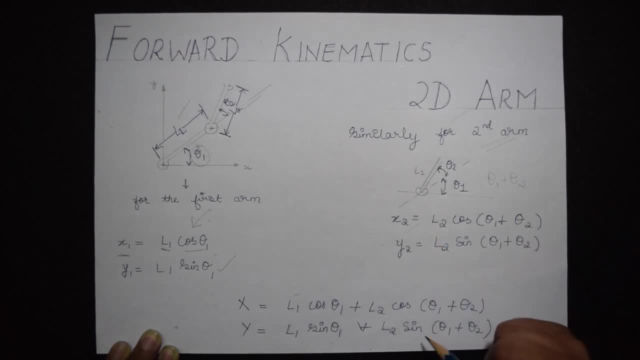 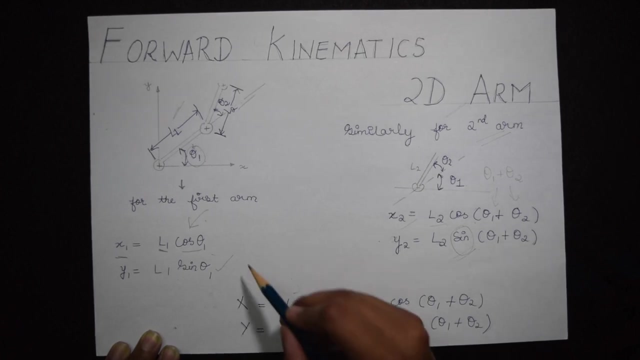 So if you want to get the x component of the second arm, you say you have L2 cos theta1 plus theta2.. And similarly, for y component, you say you have L2 sin theta1 plus theta2.. If you look at the arm as a whole, you get. 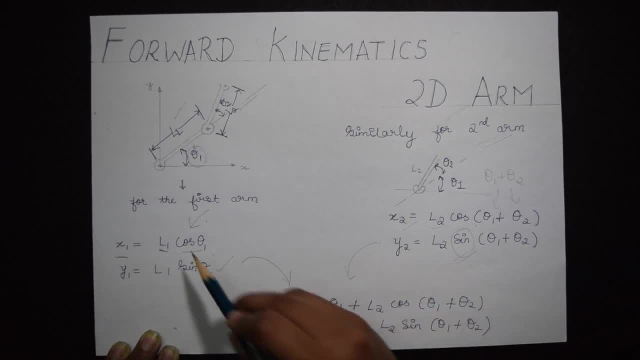 the x component of the 2D arm as the addition of x1 plus x2.. That is L1 cos theta1 plus L2 cos theta1 plus theta2.. Similarly for y you get L1 sin theta1 plus L2 sin theta1 plus theta2.. 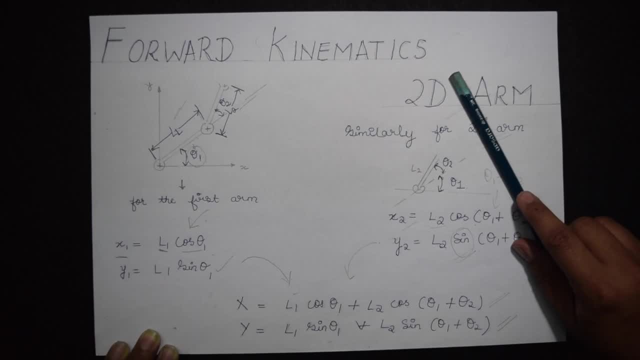 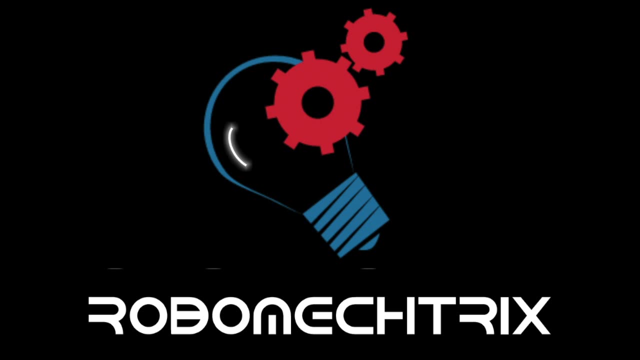 So that is all for forward kinematics of 2D arm. Later on I will teach you inverse kinematics, So for that stay tuned. Robometrics.